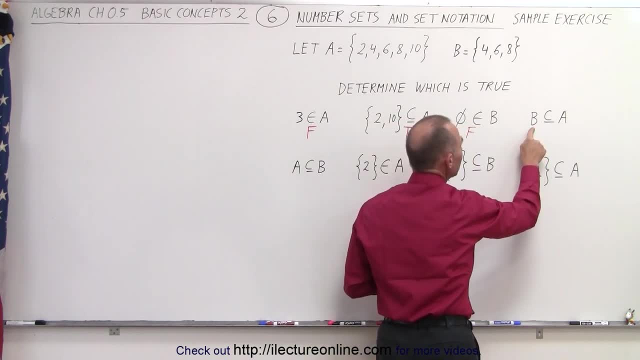 Here we're being asked or stated that B is a subset of A. That means that all the elements in B must also appear in A. So we go over here. 4,, 6,, 8 are elements of B and they all appear in the set B. 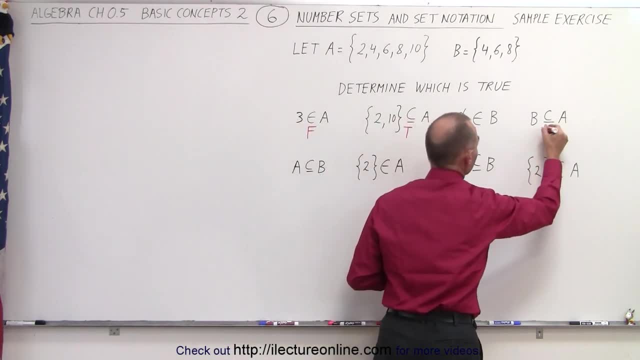 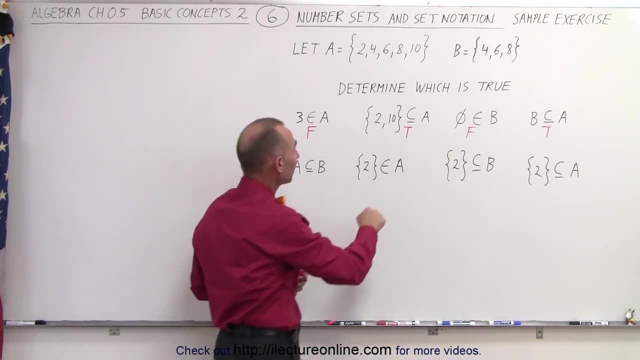 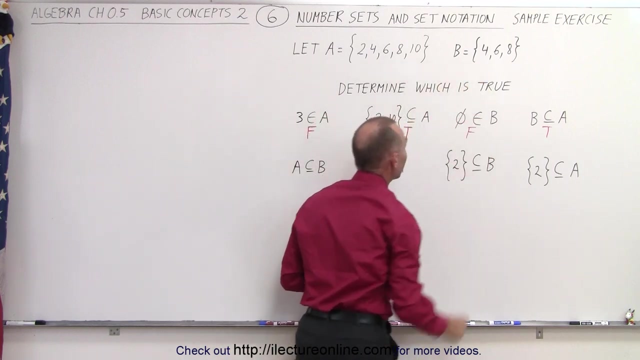 So therefore, that is a true statement Coming over here. they're telling us that A is a subset of B. Now, true that some of the elements 4, 6, and 8 that are in A also appear in B, but A has additional elements that do not appear in B. so therefore, A is basically a superset of B. 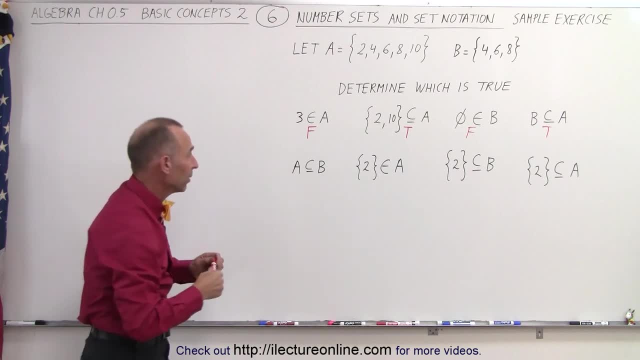 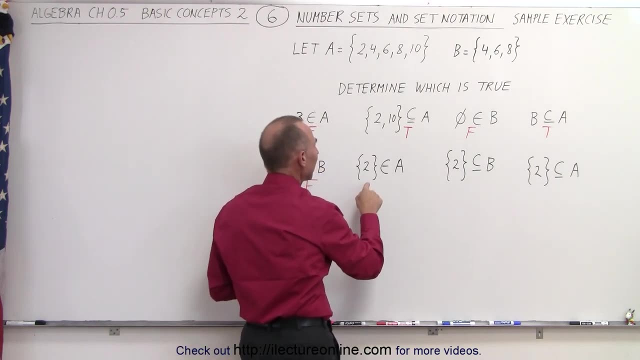 It contains all elements of B plus some more, but not the other way around. so therefore this is a false statement. here we're asked, or it's stated, that the element- not the element, but the set that contains the element 2- is an element of a. here again we have the same problem we have over here: this is a set. 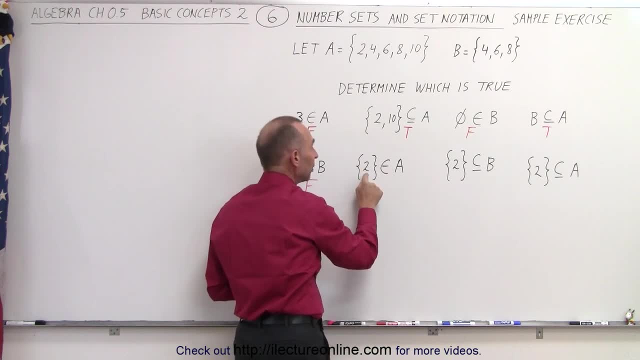 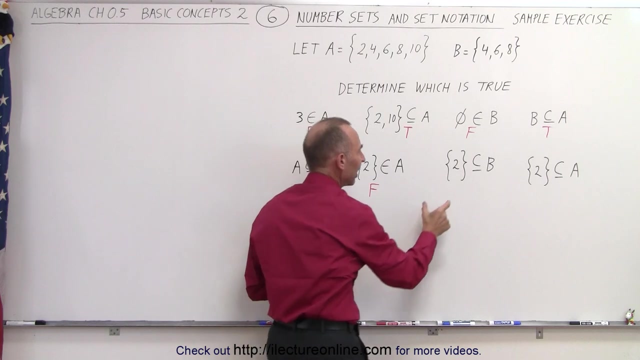 and the set cannot be an element of a, even though the element that's in the set also appears in a. so we could have said that 2 was an element of a, but not the set containing 2 is not an element of a. so this is a false statement. here the statement says that the set 2 is a subset of the. 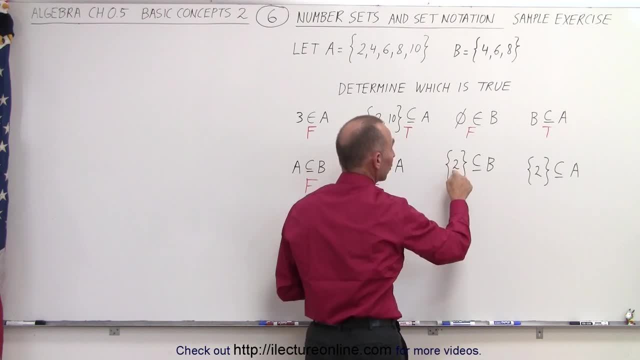 set b. now at least the dotation is correct. but this is that a true statement? we look up here and we notice that b has the elements 4, 6 and 8, but not the element 2. so therefore this cannot be a subset because it does not contain any of the elements that are in b, or i should say b does not. 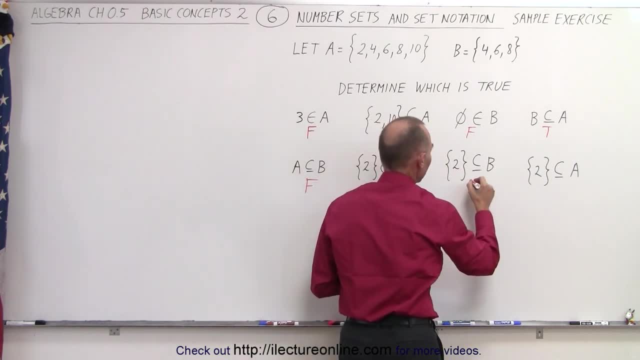 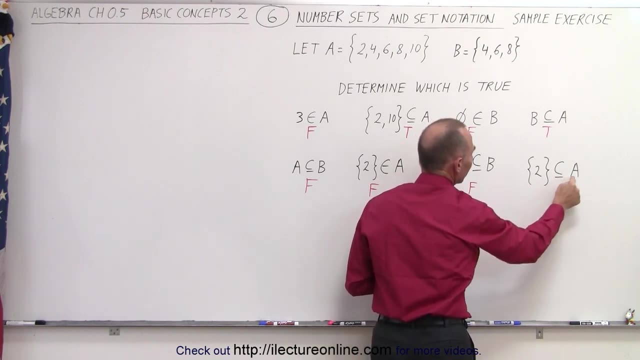 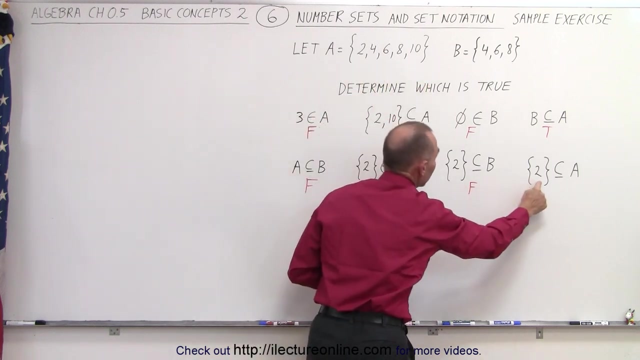 contain and the element that's in this set right here. so that's a false statement, you. and finally, the set that contains the element 2 is a subset of a. we come over here. a also has the number 2 plus some additional elements, but the element 2 does appear in a. so therefore this: 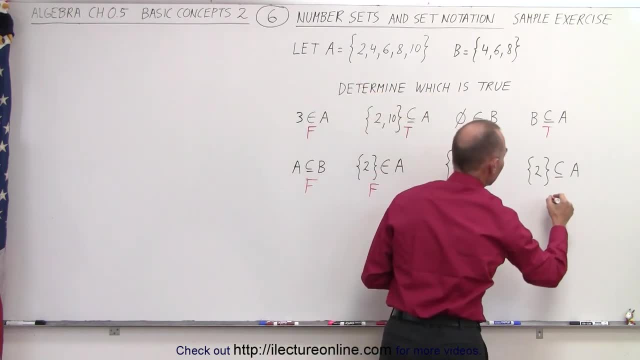 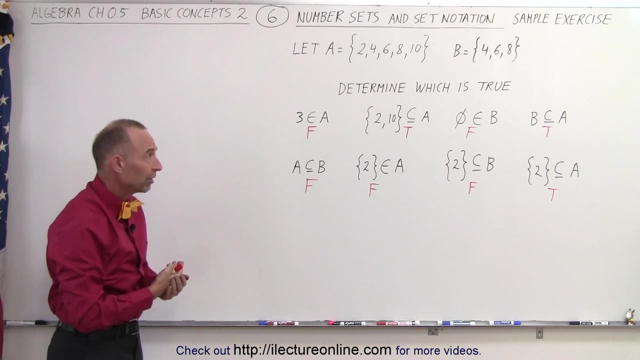 is indeed a subset of a, the correct format. so this is a true statement. so that's how we deal with the set notation. so we know when we can say something is an element of a set and we can see if something is, or a set is a subset of another set. so that's how we deal with the set notation. so we know when we can say something is an element of a set, and we can see if something is or a set, and that's how it's done.